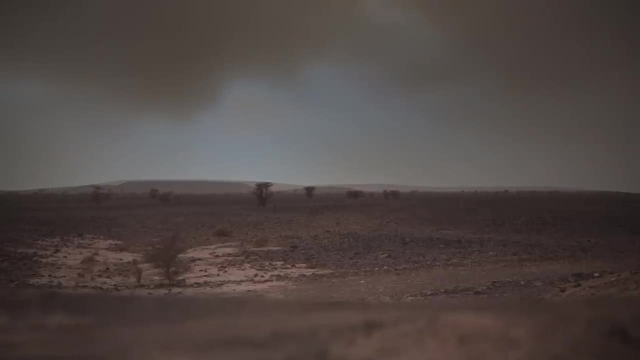 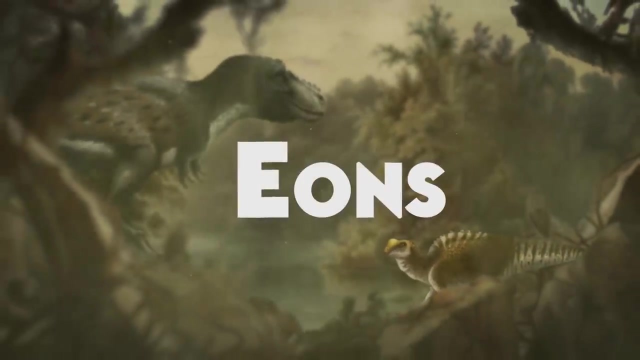 the flood deposits millions of years later. This time is known as the Carnian Pluvial Episode, and it set the stage for a new group of animals to take over the world: the dinosaurs. Evidence of just how hot and dry the world was at the start of the Triassic is trapped. 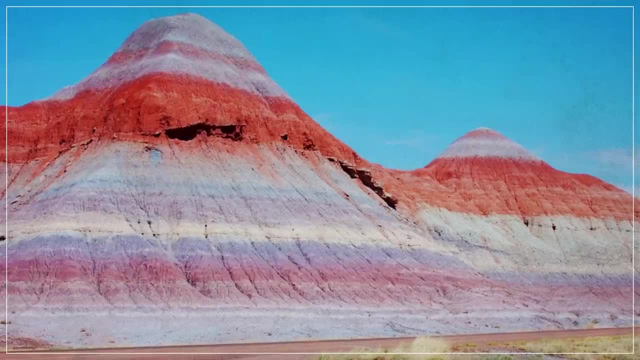 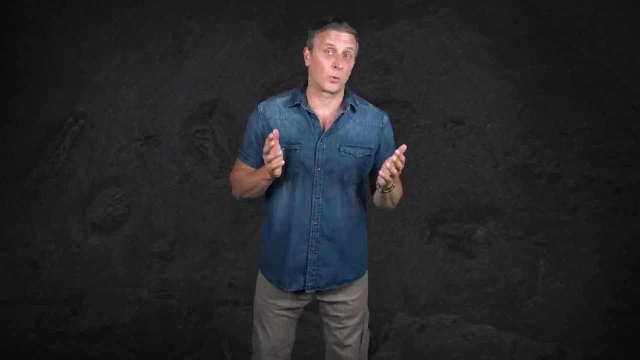 in the land beneath our feet. Rocks from that period are mostly swathes of red sandstone and soil deposits from dry woodlands, with no sign of the coal swamps that had covered the world during much of the Permian. And one major reason that the world was so dry was the shape of Pangea With all the continents locked together, rain clouds couldn't move much past the coastlines and there were no big mountain ranges to break up the low, arid land. Now, dinosaurs did exist in this dry post-Permian world, But they didn't have the ability to. 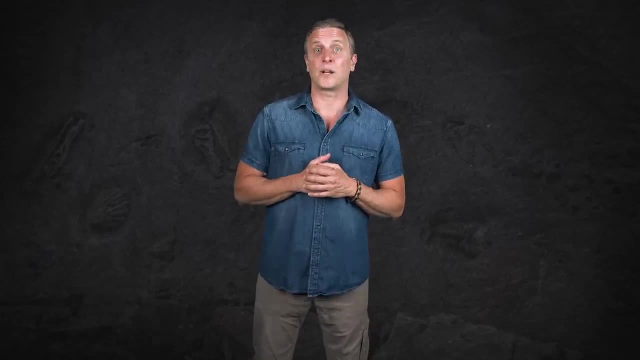 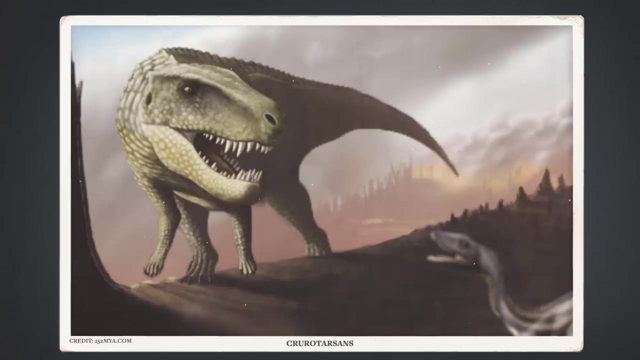 survive. They were still vying for their place among the early reptiles and reptile-like mammal ancestors. The dominant carnivores back then were the early Crubotarsans, a broad group of croc-like animals that included reptiles like Pseudosuchians and Phytosaurs. For example, there was Ornithosuchus. 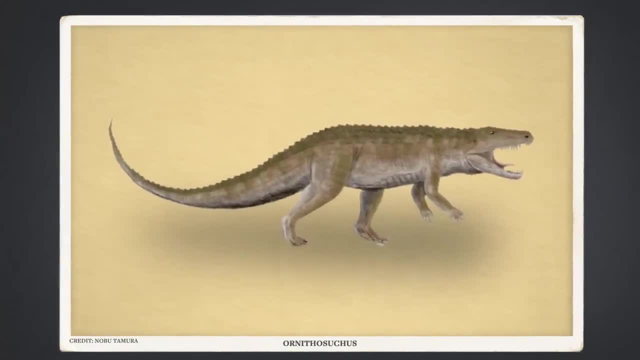 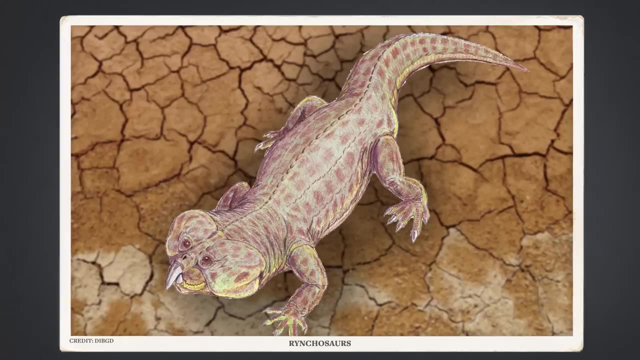 which had long hind legs and could actually stand up when it wanted to run, which I imagine would have been both awesome and terrifying to actually see. But even stranger than these were the Rhynchosaurs, herbivores with parrot-like beaks and sometimes. 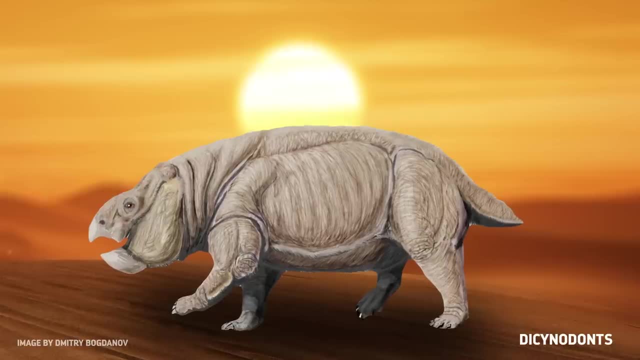 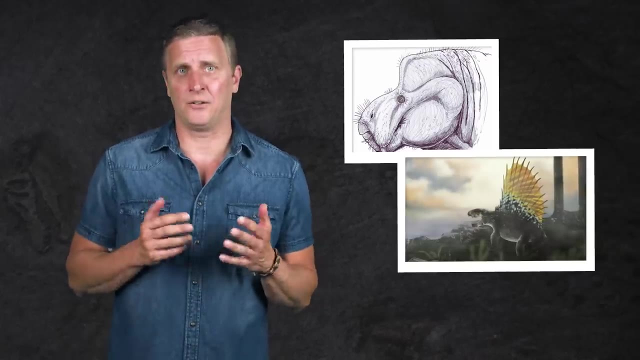 cheekbones to die for all in a chubby lizard body. And although there were no true mammals, there were Dicynodonts, the closest things to them at the time. They were actually more closely related to us than, say, Dimetrodon, despite being scaly four-legged creatures. 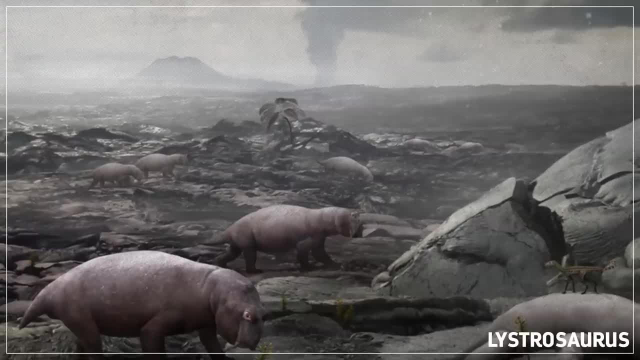 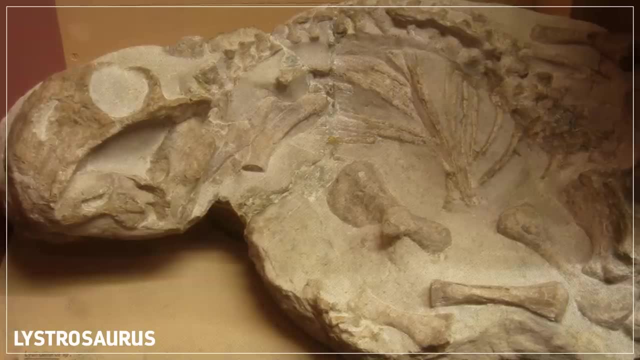 with bills and tusks. All of these fascinating creatures were widespread for most of the Triassic, with one species of Dicynodont called Lystrosaurus being so common all over the world that its fossils were actually used to help construct the idea of plate tectonics. 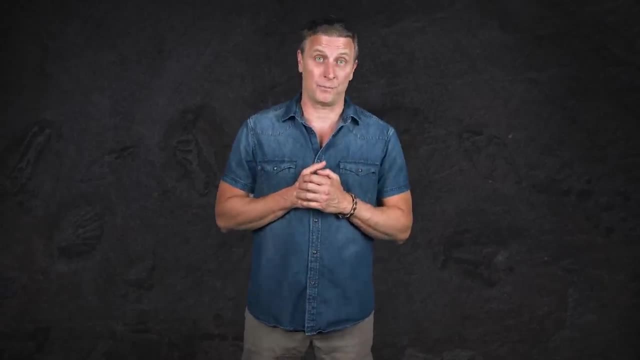 But these animals, adapted as they were for life in a dry climate, were in for a big shakeup. Most of what we know about the history of climate comes from plant fossils and rock types, And in the early 1990s, two British geologists 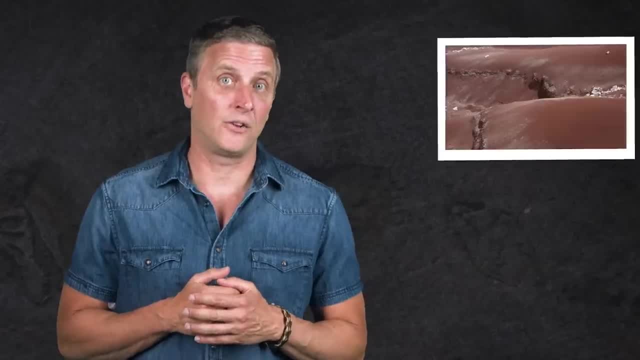 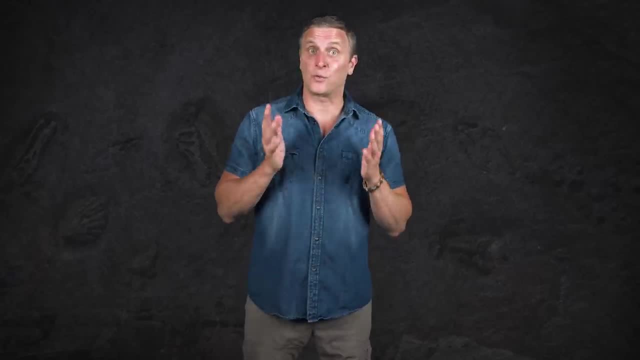 didn't match the dry climate of the Triassic that they knew. Instead of finding red, slowly deposited sand, they found thick layers of river rocks, sediments from giant lakes and evidence of coal swamps. All of these were signs of massive rainfall over the course. 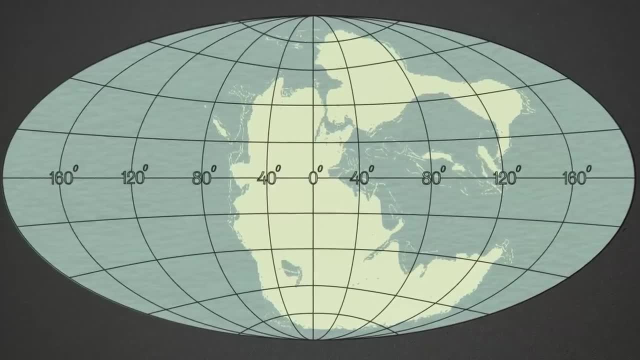 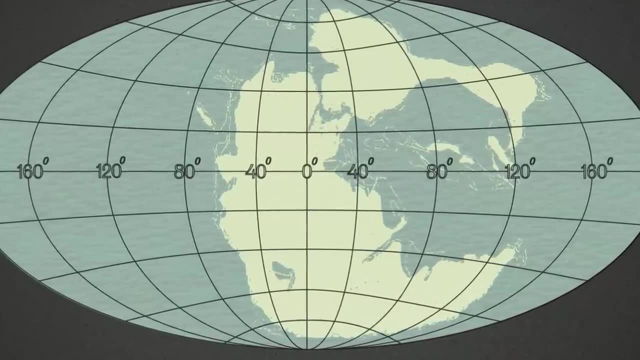 of some two million years. But, stranger still, these traces of a suddenly wet climate turned out to be everywhere, from England to the Americas, to Israel and regions that were far apart at the time. That meant that the rise in rainfall must have been worldwide. 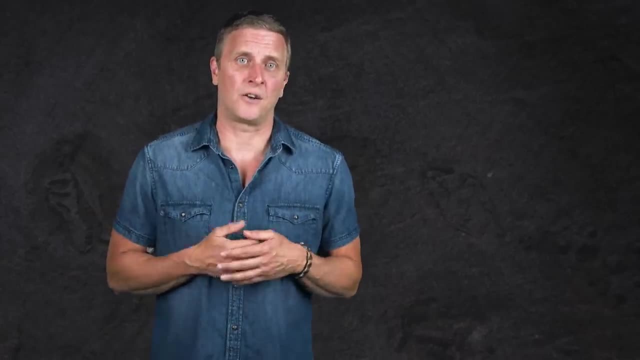 Initially, other geologists were skeptical: Couldn't these rocks just be explained by a lot of big local floods? Well, over the next two decades, reports of more and more weird rocks kept trickling in, And they kept pointing to a world that 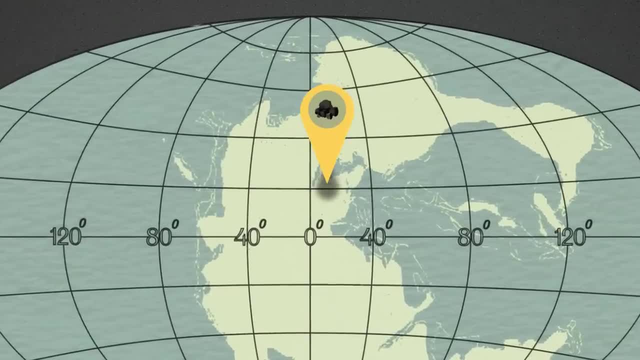 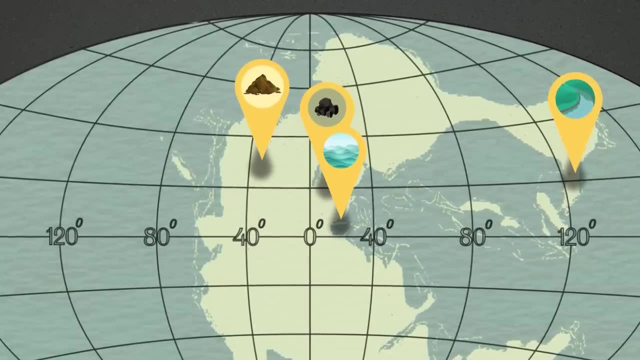 was getting wetter and wetter. The rocks revealed coal deposits in Austria, traces of ancient lakes in Italy, wet soils in Utah and giant rivers in China. And they all dated to the same window of time, between 232 and 234 million years ago. 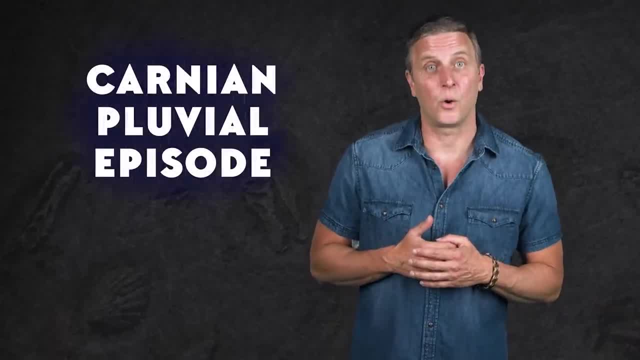 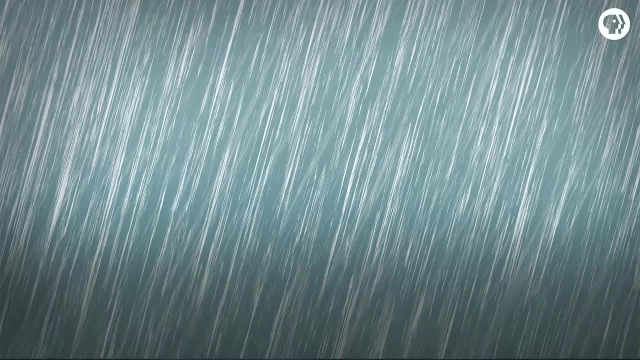 In time, this phenomenon came to be known as the Carnian Pluvial Episode, or CPE. The Carnian is the name of the geologic age within the Triassic. when all this happened, And for what it's worth, I seriously thought about naming this episode the Chronicles of Carnia, But I didn't because that would have been dumb. And pluvial means rain, and it rained a whole awful lot. For example, one estimate suggests that average annual rainfall in what's now Utah almost quadrupled, reaching a peak of 1,400 millimeters, or about 55 inches of rain a year. For context, that's how much a temperate rainforest gets today, like, say, in the Pacific Northwest, And this would have happened over, and, over, and, over and over again all around the world. It was not one big flood, It was more like floods every year, all over the place for two million years. But things were bound to change, And one of the biggest changes was the sudden abundance of dinosaurs In rock data to the start of the Carnian Pluvial episode. dinosaurs account for about 5% of the fossils of terrestrial vertebrates. 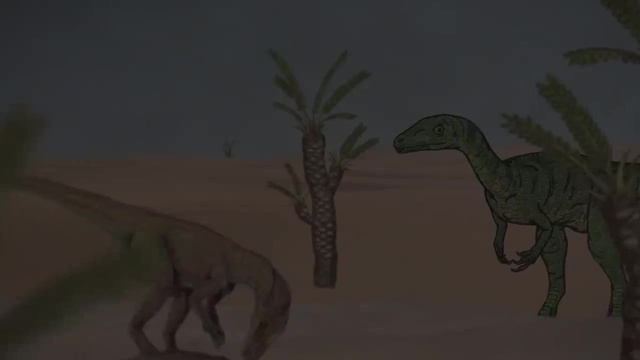 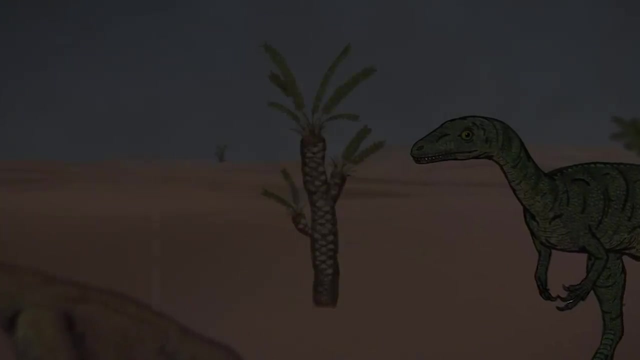 But by the end they make up more than 90% of those fossils. So what made the dinosaurs so suddenly successful? Were they better off than their competitors in this newly-wet world? Or did other animals simply die, leaving them to rule the world by default? 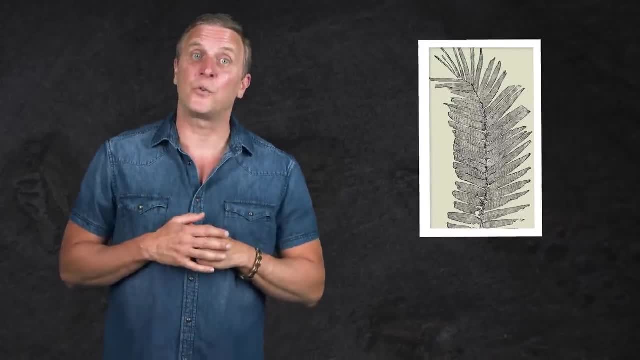 The key might not have been the rain itself, but what the rain brought with it: A proliferation of giant plants. During this time, we begin to see lots of large conifers and big corals, And that's when we begin to see a lot of giant plants. 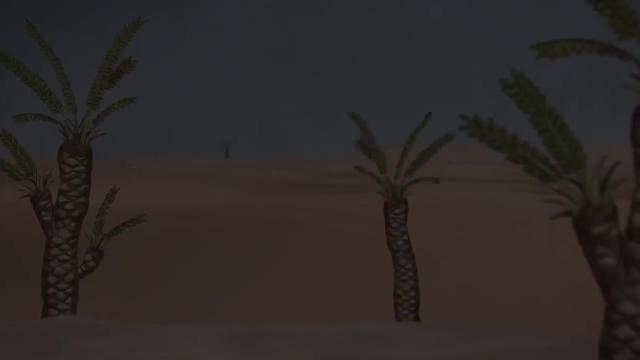 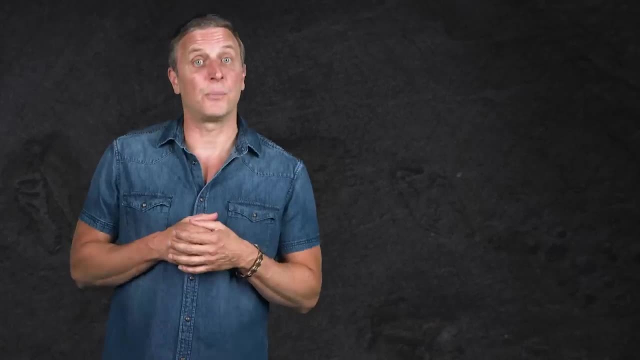 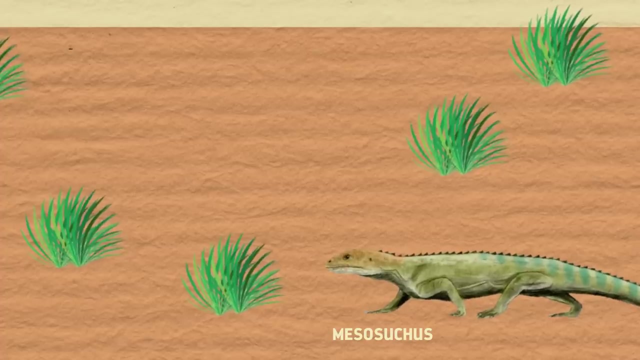 And for herbivores, this change in food supply could have been a game-changer. For example, rhynchosaurs were abundant, but they were also short And they couldn't stand on their hind legs to reach higher leaves. This would have been fine in a dry environment where plants tend to stay close to the ground. 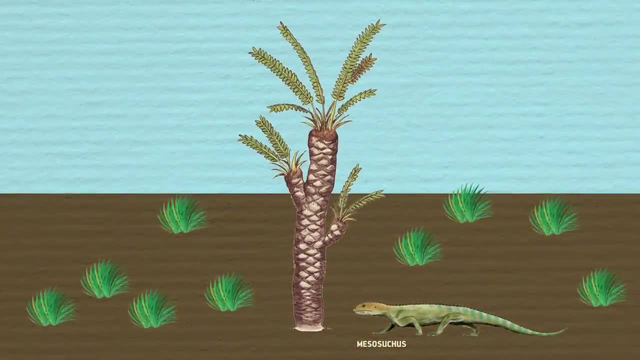 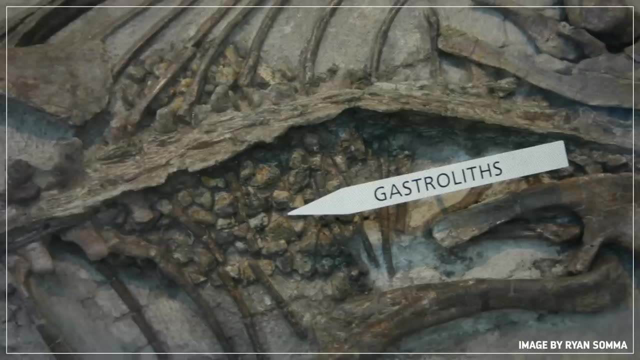 But in a wet forest, rhynchosaurs would only have been able to eat smaller plants or whatever leaves and fruit fell to the ground. Meanwhile, the cynodonts were herbivores too, But they didn't have teeth, And they also didn't use gastroliths, the rocks that some animals like birds swallow. 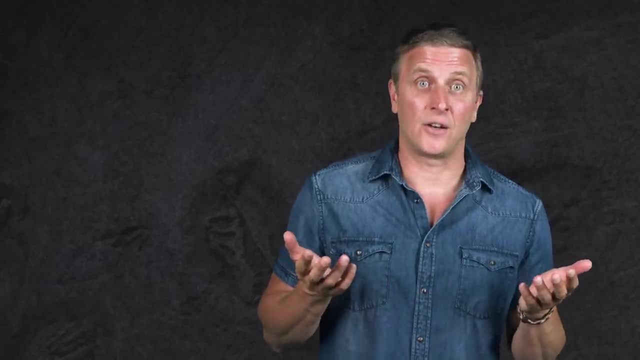 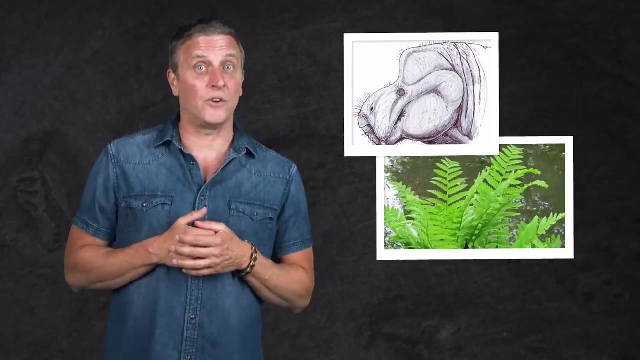 to help digest plant material. Without teeth or gastroliths, the cynodonts would have had a hard time eating anything fibrous like wood. And sure enough, fossils of the cynodont poop from this time have been found to contain mostly soft ferns with only small amounts of wood. 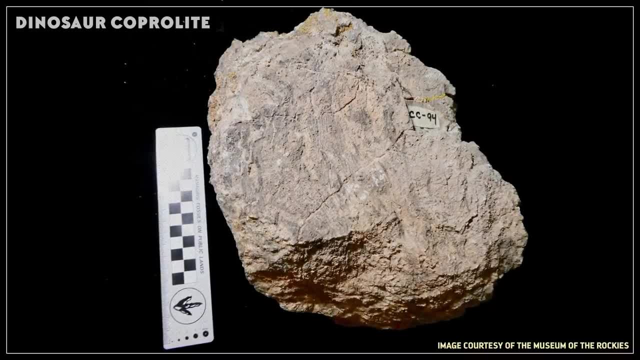 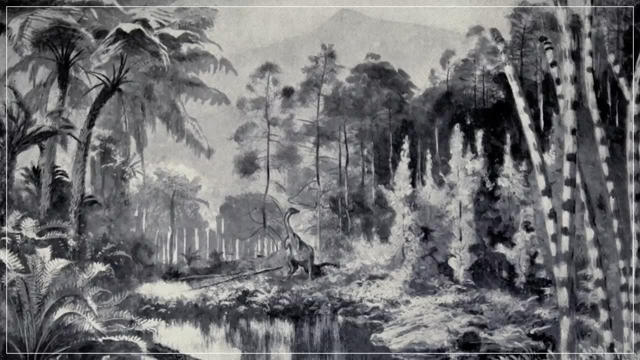 By comparison, some plant-eating dinosaurs, which both had teeth and used gastroliths, left us poop fossils that are up to 85% wood, which is a lot of fiber. So as the climate became wetter, soft, small ferns were quickly replaced by tall woody. 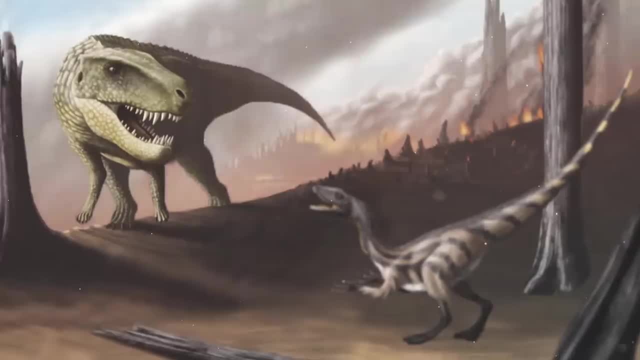 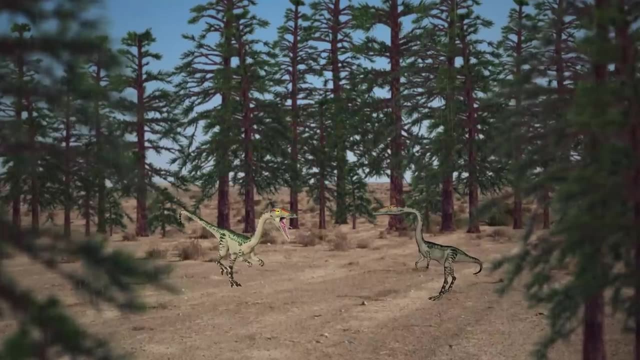 conifers, which the cynodonts and rhynchosaurs didn't eat, And without rhynchosaurs and the cynodonts, even the carnivores, those crurotarsans would have lost a lot of their food supply. So maybe, instead of being better adapted to this new environment, dinosaurs were just 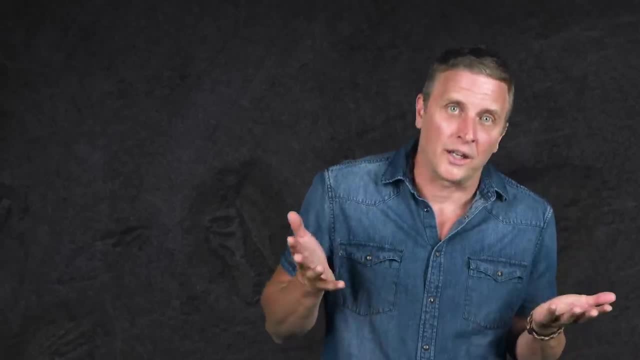 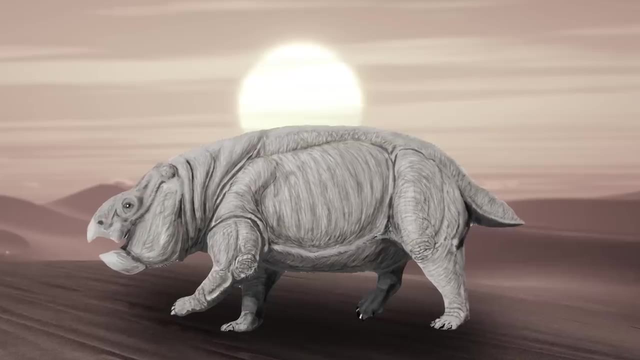 the only major group of reptiles left standing or, you know, squatting. Even though we don't know exactly why the rain helped the dinosaurs, we do know that dinosaurs became a lot more abundant during the Carnian Pluvial episode. And then the cynodonts, the rhynchosaurs and many of the early crurotarsans soon went extinct. Now there's still the question of what made it rain for two million years in the first place. Well, right before, the rains came some 235 million years ago. 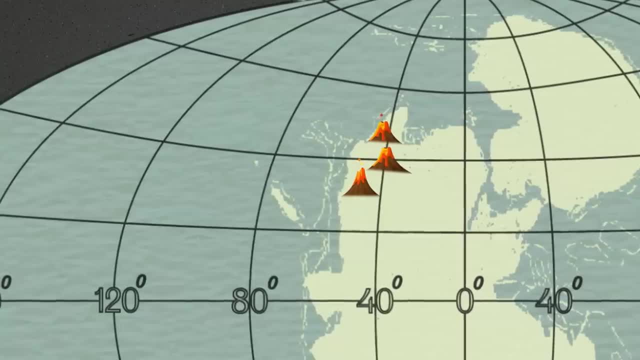 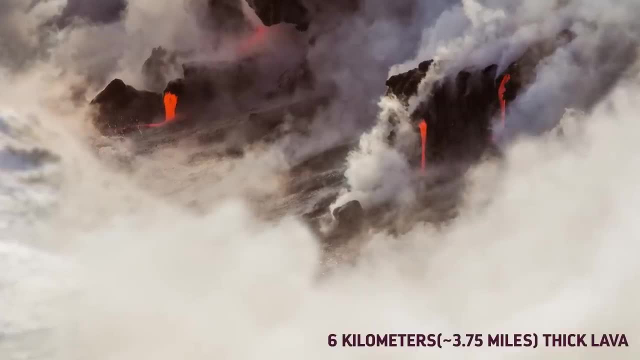 there was a huge burst of volcanic activity in Alaska and British Columbia. Today it's known as the Rangelian Eruptions. These eruptions lasted for more than five million years, churning out a layer of lava that got to be six kilometers thick and releasing enough CO2 to raise temperatures by about. three to ten degrees worldwide And over a very long time. warmer temperatures can create a wetter climate because they can speed up the water cycle, driving more evaporation of surface water into the atmosphere, among other things, And in fact, because of this increase in atmospheric moisture, the CPE is also sometimes called. 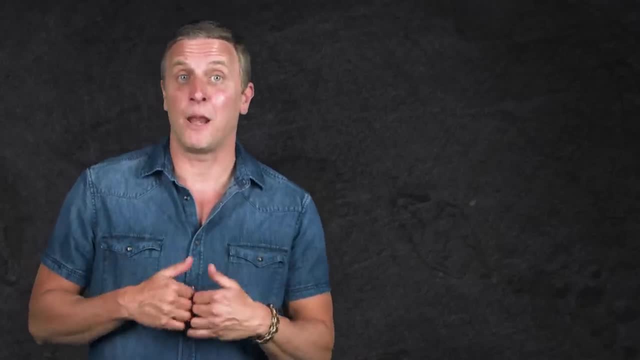 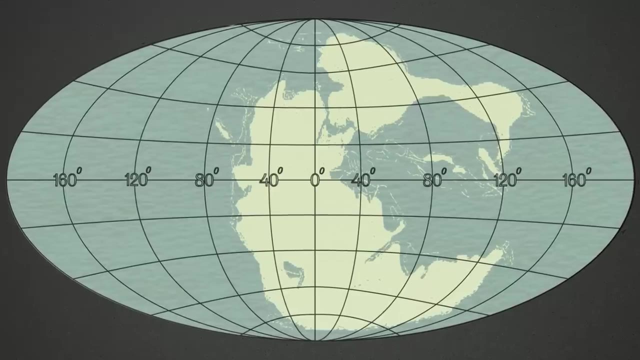 the Carnian Humid Episode. But for what it's worth, my personal favorite name for this episode is called the Wet Intermezzo, which I just think is delightful, so let's try to bring that term back, okay. Anyway, after about a million years of these eruptions, the atmosphere became so warm and 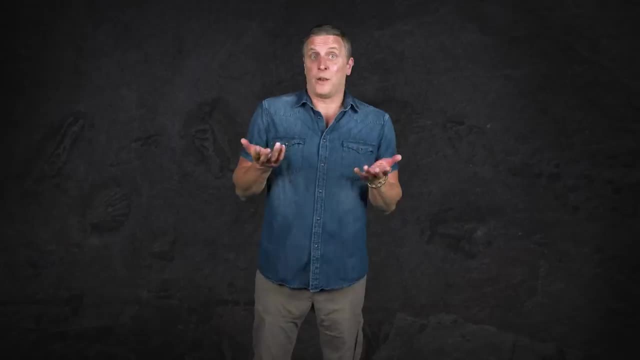 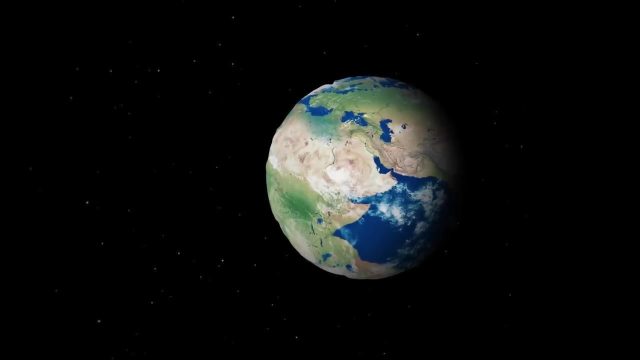 wet. that rain could finally reach even Pangea's vast interior. Okay, but then how did it stop? Well, when carbon levels are really high for a really long time, our planet can be pretty good about getting some of the extra carbon back into the ground, where it belongs. 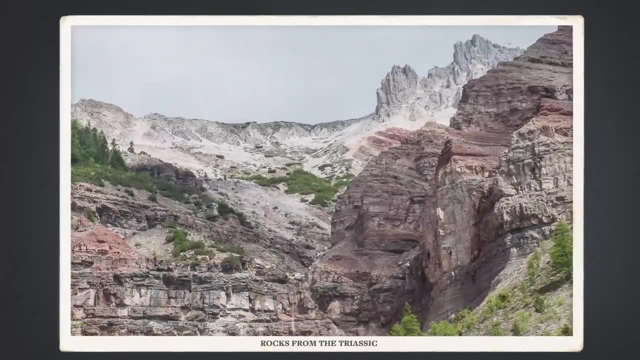 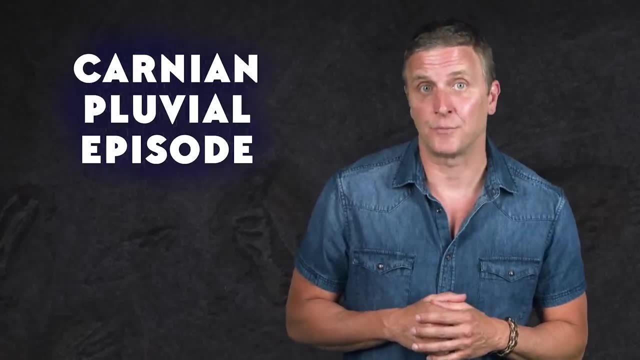 Plants take it in and store it in their tissues. Weathering and eroding rocks absorb it and the oceans soak it up to form carbonate rocks like limestone. So, as the Rangelian eruption slowed down, the carbon cycle was eventually able to stabilize. 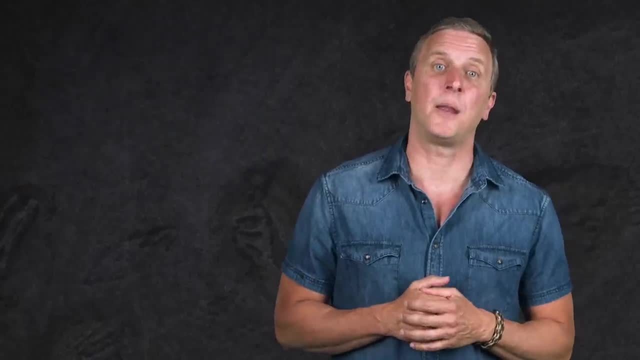 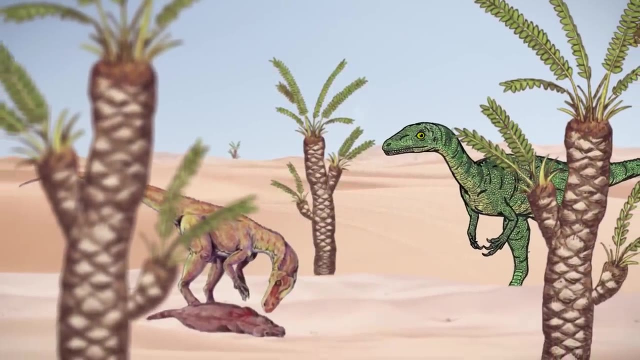 Excess CO2 was reabsorbed from the atmosphere and the CPE gradually came to an end. By the time the eruptions had completely ended 230 million years ago, the world had returned to a classically hot, dry Triassic climate. that only ended when Pangea began to break. 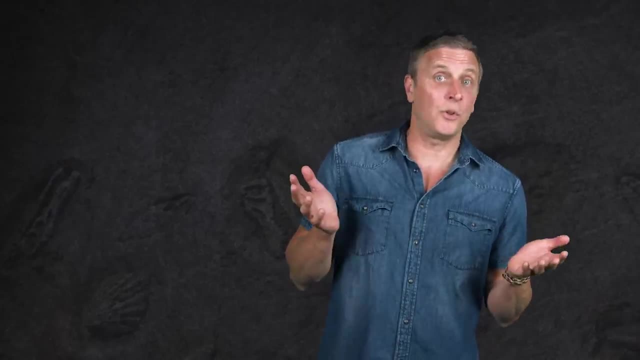 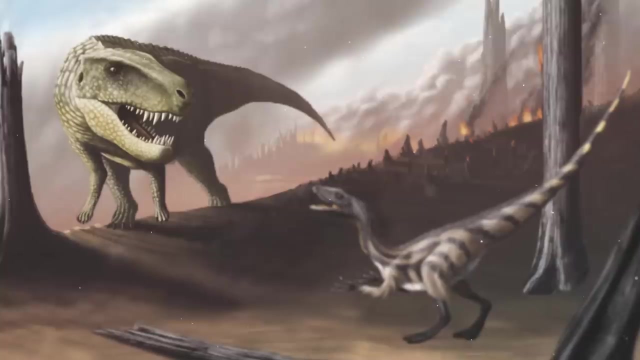 up. But even though the Carnian Pluvial Episode was short, only 2 million years, its impacts on life were permanent. All that rainfall helped conifers spread and diversify, leading to the pine trees that we know today. And while the start of the Triassic may have been the land of weird croc-like, 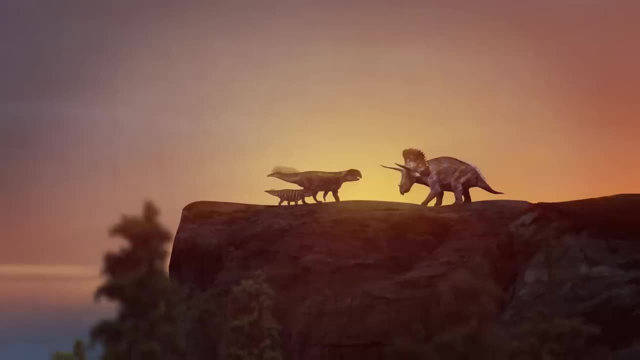 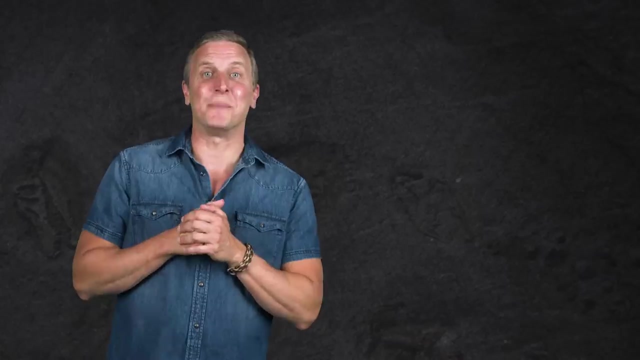 things running around in their hind legs. by the time the rains ended, the world had fully entered the age of dinosaurs. Thanks for joining me for this wet intermezzo Now. wouldn't you like to have all of natural history right there on your wall? 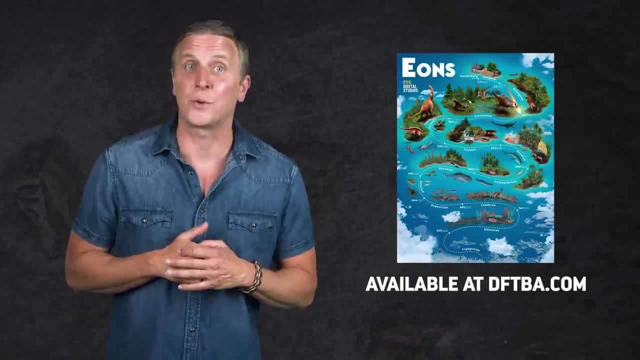 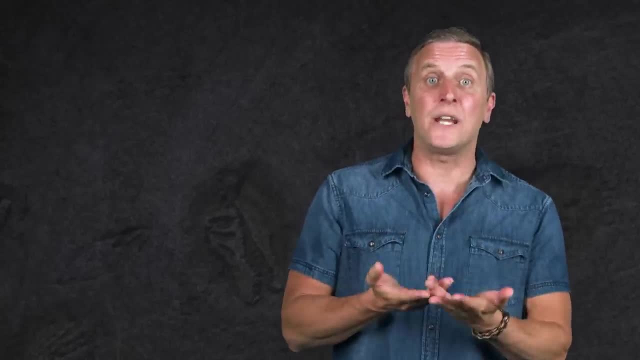 I would, And now you can, with the first ever Eons poster created by Franz Anthony. Just go to DFTBAcom and links are in the description, And let me know what you want to learn about, because you know by now that we read your. 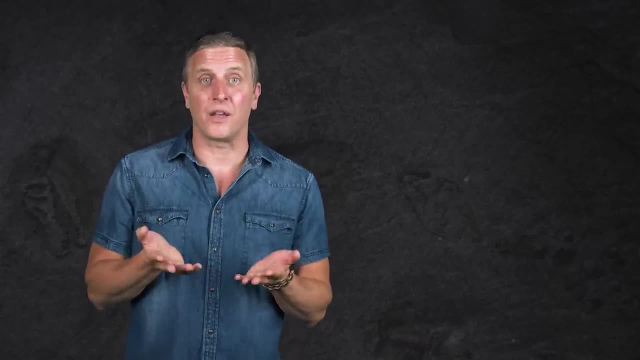 comments. And if you haven't already- and I don't know why you wouldn't have, but if you haven't- you should go to youtubecom, slash eons and subscribe. Thank you.